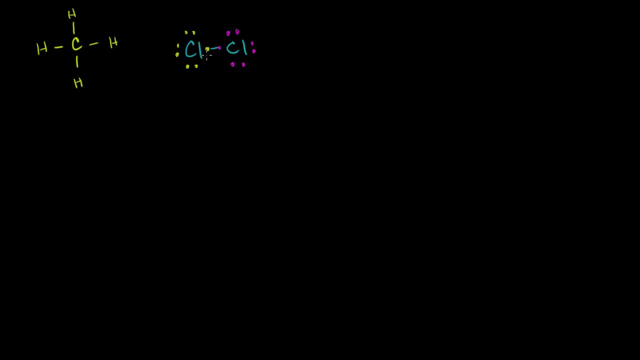 these chlorines, this bond's just going to break. Each of these chlorines are just going to take their part of the bond. So this guy on the left, he's just going to take his electron and notice I draw it with this half. 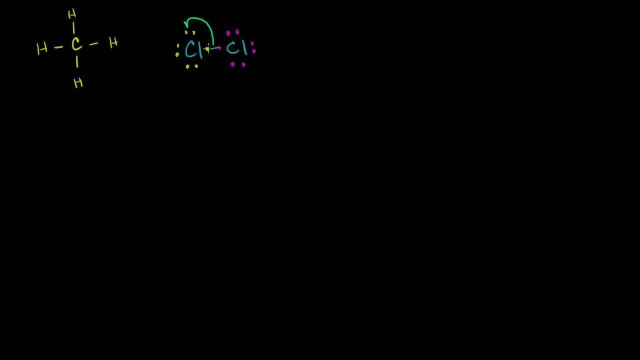 arrow. It looks like a fish hook. It's just half an arrowhead. This means that this electron is just going to go back to this chlorine and this other magenta electron is going to go back to the right chlorine. So we could draw it like that. 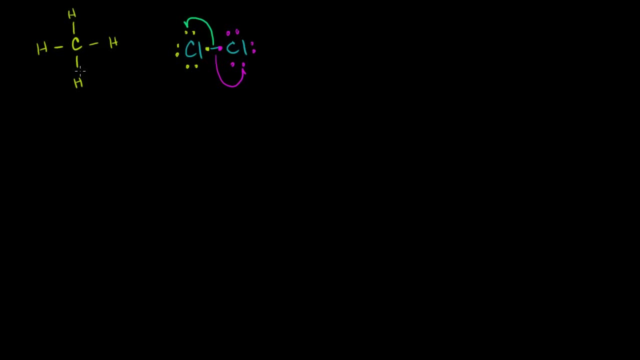 If it was up to me, I would have drawn it more like this to show that that electron just goes back to the chlorine. But the convention shows that you could show that half of the bond is going back to the entire atom, The entire atom. 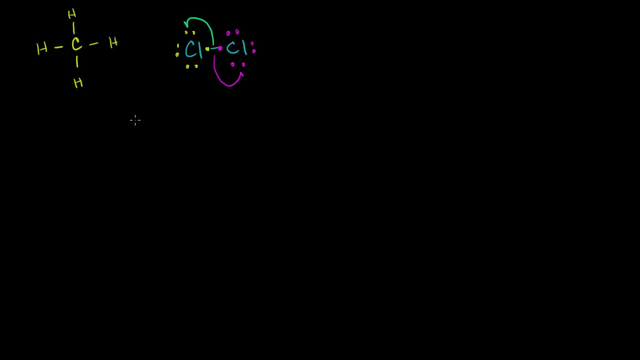 Now, after this happens, what will everything look like? Well, we're still going to have our methane here. It hasn't really reacted, So we still have our methane. Let me draw it a little bit. So we still have our methane here. 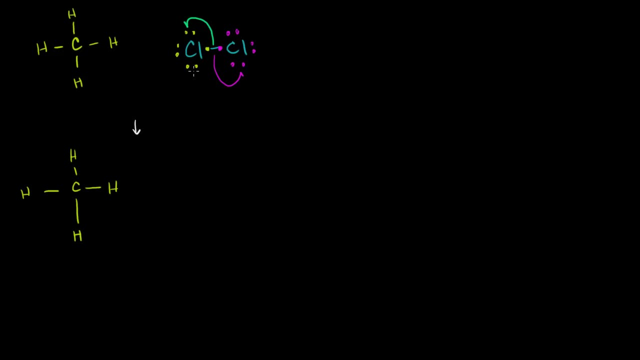 And all that's happened because we've put energy into the system. we've been able to break this bond. The molecular chlorine has broken up into two chlorine atoms, So we have the one on the left over here, We have the one on the left. 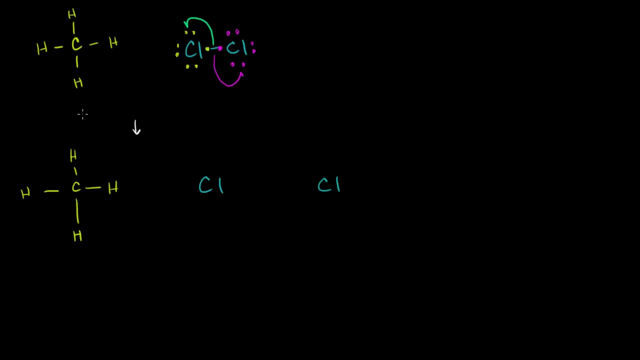 We have the one on the right, We have the one on the left, We have the one on the left, We have the one on the left over here, And then we have the one on the right, And let me draw the left. valence electrons. 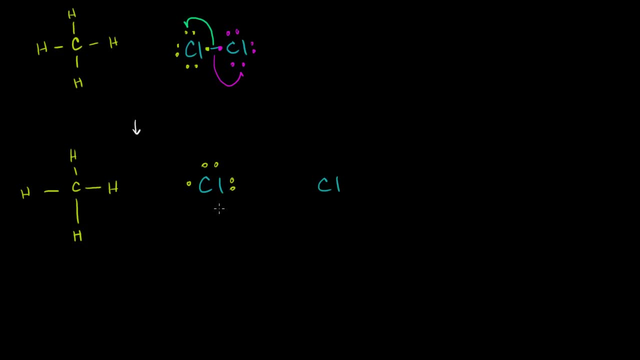 It has 1,, 2,, 3,, 4,, 5, 6, 7.. I just flipped it over so that the lone electron is on the left-hand side, right here, And then you have the guy on the right. 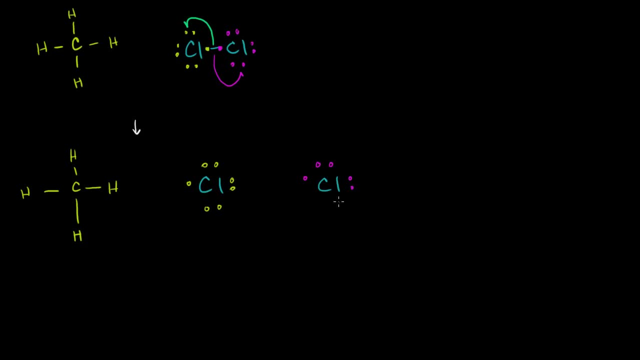 He has 1,, 2,, 3,, 4,, 5,, 6, 7 valence electrons. Now that each of these guys have an unpaired electron, they're actually very, very, very reactive and we actually. 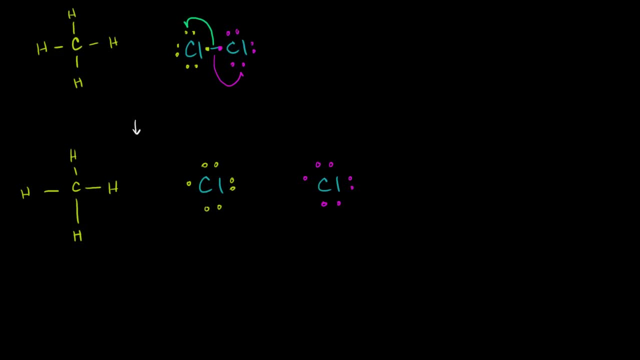 call any molecule that has an unpaired electron and is very reactive a free radical. So both of these guys now are free radicals And actually the whole topic of this video is free radical reactions. Both of these guys are free radicals And you've probably heard the word free radical before in the 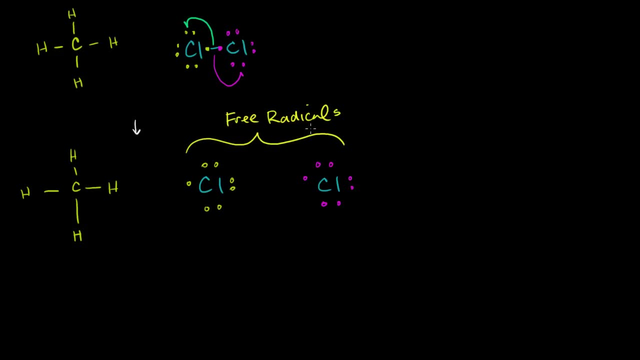 context of nutrition that you don't want free radicals running around, And it's the exact same idea. It's not necessarily chlorine that they're talking about, but they're talking about molecules that have unpaired electrons. They'll react with some of the stuff. 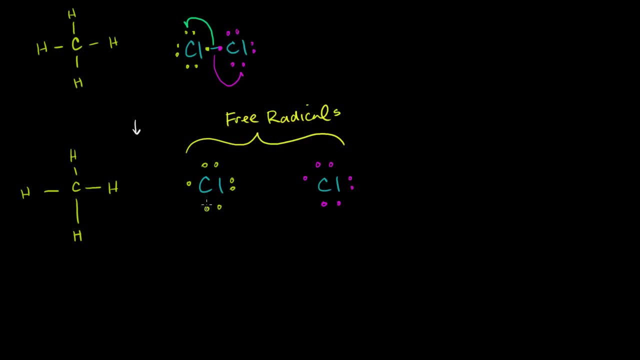 Your cell's machinery, maybe even with your DNA, maybe cause mutations that might lead to things like cancer. So that's why people think you shouldn't have free radicals in your body. But as soon as we form these free radicals and this step right here where we put energy in the system, 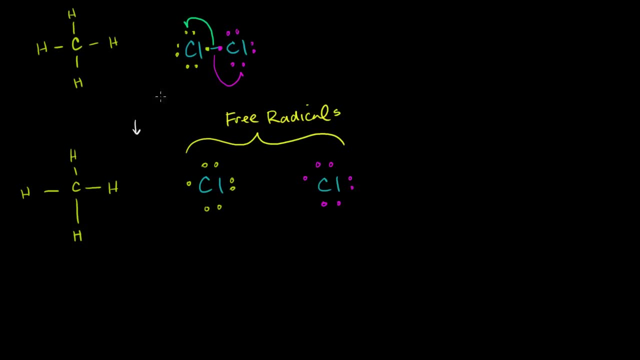 to break this bond. we call this the initiation step. Let me put this: We used energy here. This was endothermic. We used energy. This, right here, is the initiation step, And what we're going to see in general with free radical reactions is: you need some energy. 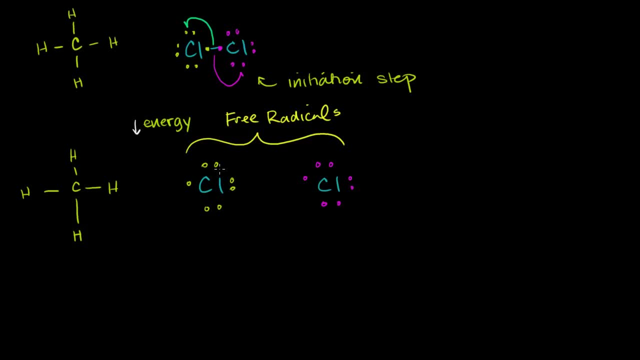 to get it started. But once it gets started it kind of starts this chain reaction And as one free radical reacts with something else, it creates another free radical And that keeps propagating until really everything has reacted. And that's why these can be so dangerous, or so. 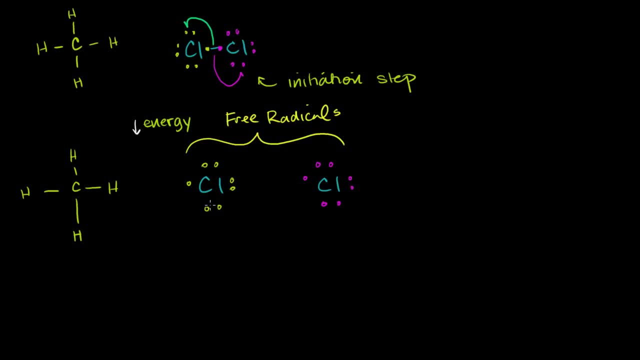 bad for biological systems. So I've told you that they react a lot. So how will they react now? Well, this guy wants to form a pair with someone else And maybe, if he swipes by this methane in just the right way. 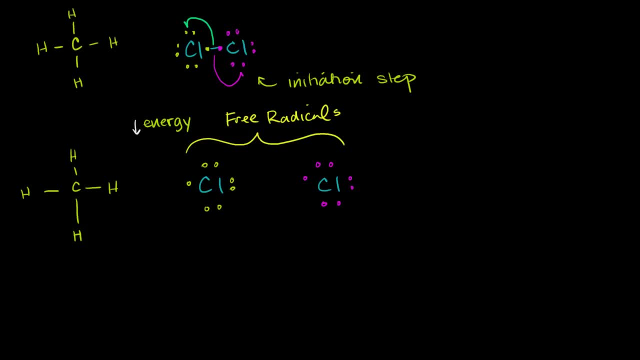 with just enough energy. Let's see. Let's see. What will happen is he could take the hydrogen off of the carbon, And not just the proton, the entire hydrogen. He will form a bond with the hydrogen using the hydrogen's electrons. 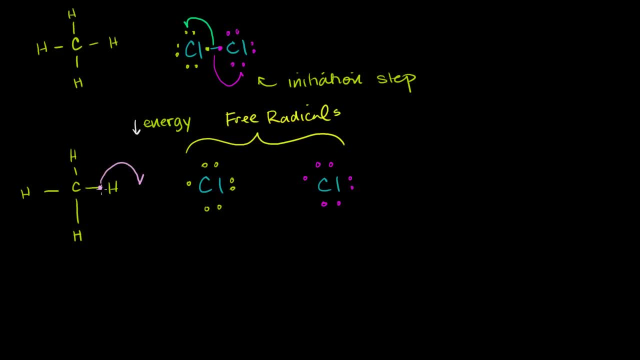 So they'll get together and they'll form a bond. The hydrogen will contribute one electron. Notice I'm drawing the half arrow again. So the hydrogen isn't giving away the electron to someone else. that would be a full arrow. The hydrogen is just contributing its electron. 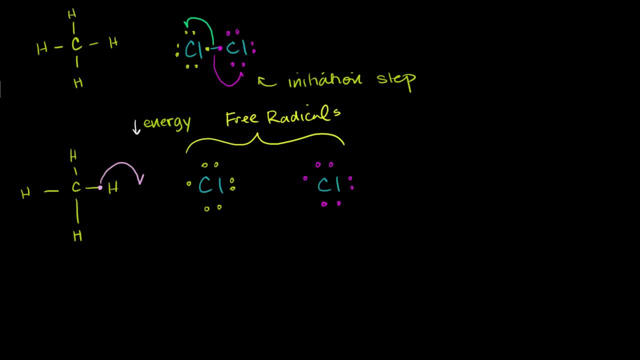 to half of a bond, And then the carbon would do the same. I'll do that in blue. So the carbon, this valence electron right here, could be contributed to half of a bond, And then they will bond And this bond over here will break. 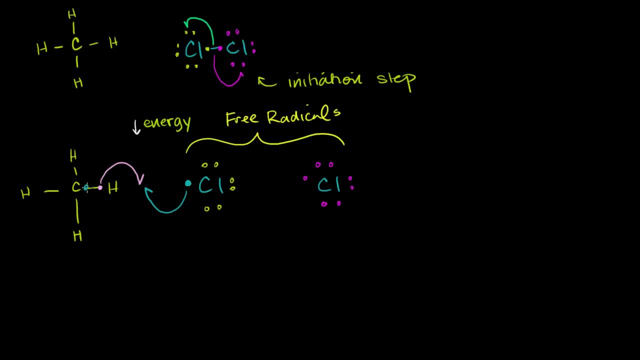 And so the carbon over here on the left, this carbon over here, will take back its electron. So what does everything look like after that's done? So our methane now it's no longer methane, It is now, if you think about it. so we have three hydrogen. 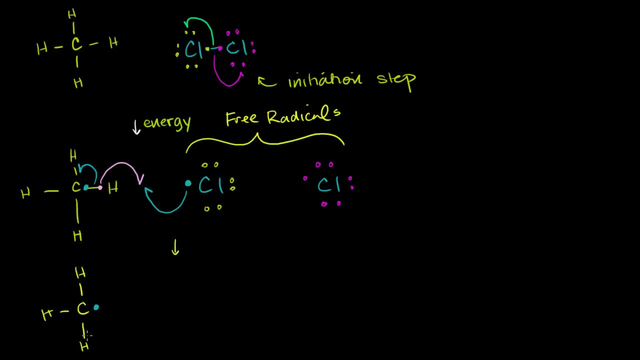 It took its electron back. It is now a free radical. It now has an unpaired reactive electron. The hydrogen and this chlorine have bonded, So let me draw the chlorine. It has this electron right over here. It has the other six valence electrons. 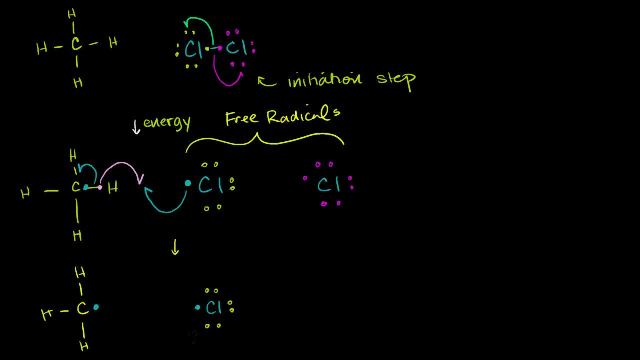 One, two, three, four, five, six, And we have the hydrogen. We have the hydrogen with its pink electron that it's contributing to the bond. And so we have the hydrogen, And so we have the hydrogen with its pink electron that it's contributing to the bond. 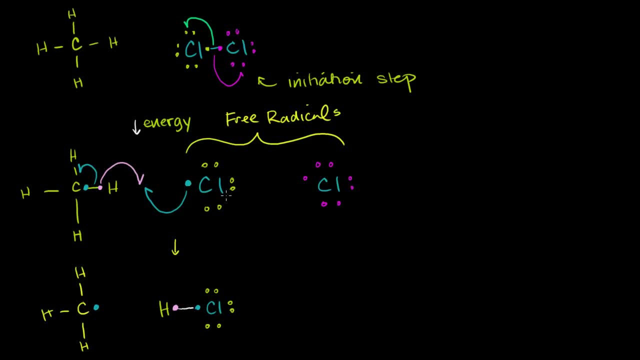 So we have them bonded. now This chlorine is no longer a free radical, although this one out here is still a free radical. Let me copy and paste it. So it's just hanging around, Copy and paste, And now notice we had one free radical react. 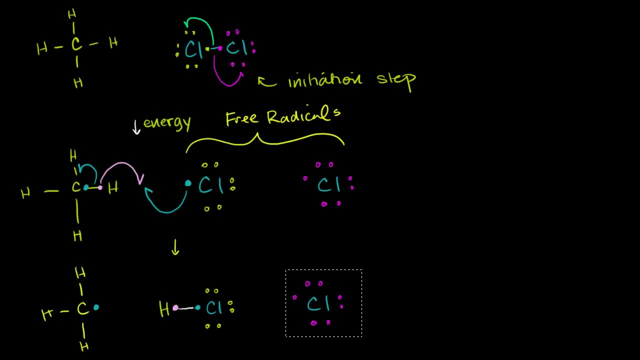 but it formed another free radical, And that's why we call this a propagation step. We call this a propagation step. So this right here is a propagation, Propagation step. When one free radical reacts, it created another free radical. Now, what's that free radical likely to do? 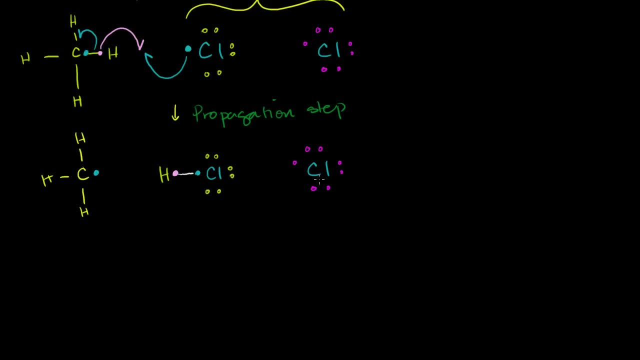 You might be tempted to say, hey, it's going to just react with that other chlorine. But think about it. These molecules, there's a gazillion of them in this solution. So the odds that this guy is going to react exactly with that other free radical. 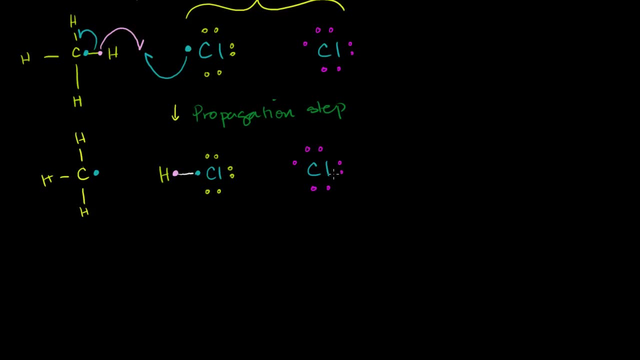 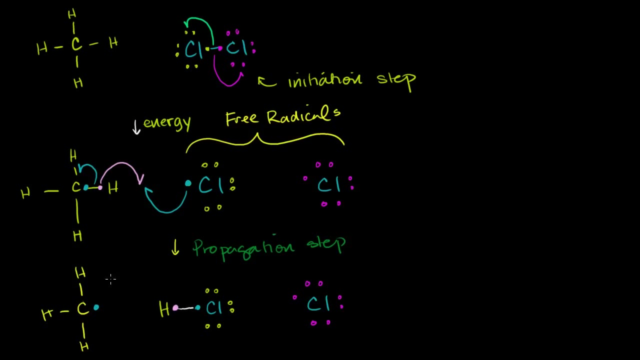 is actually very low, especially early on in the reaction where most of the molecules are still either methane or molecular chlorine. But this guy is much more likely to bump into another molecular chlorine than he is to bump into one of these original free radicals that. 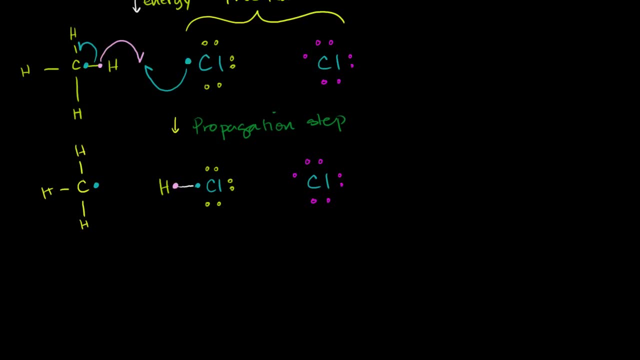 formed. So if he bumps into another molecular chlorine in just the right way. so let me draw another molecular chlorine. So that's another molecular chlorine And each of these: 1, 2, 3,, 4,, 5,, 6, 7,. 1, 2,, 3,, 4, 5,, 6, 7,. 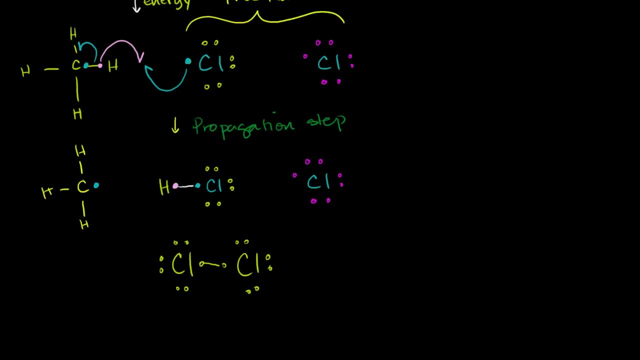 there is a bond here. If they bump in just the right way, this chlorine, this chlorine electron might get contributed And this free unpaired electron will be contributed, can get contributed. And then this CH3, I guess we could call it this free radical. 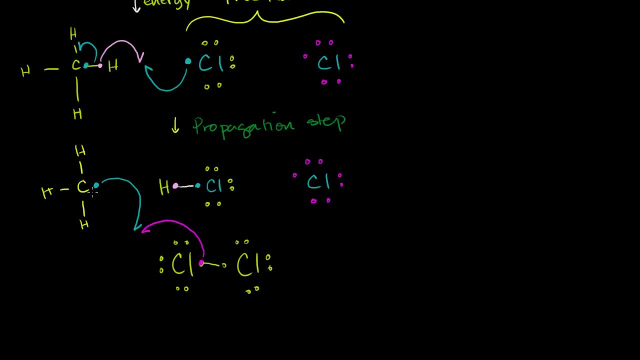 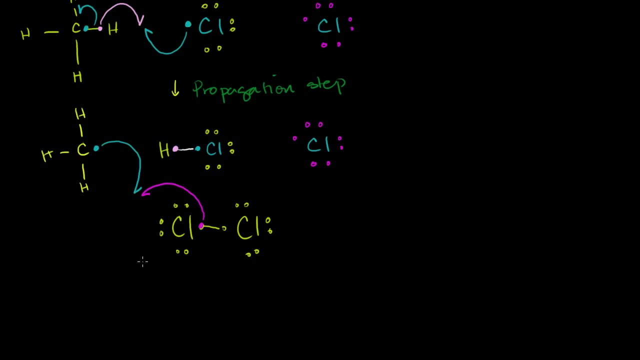 this carbon-free radical or this methyl-free radical will then form a bond with this chlorine, And what's everything going to look like after that? Well, after that happens, this is now bonded to a chlorine. It's now chloromethane. 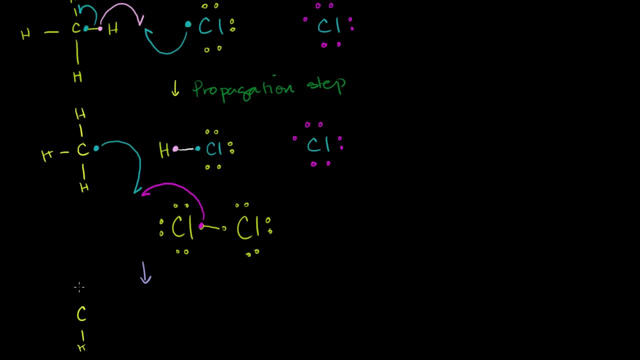 Let me draw it. So it's carbon hydrogen, hydrogen, hydrogen. Now it's bonded to a chlorine. Let me draw the electrons so we can keep track of everything. We have that magenta electron right over there, And then we have the chlorine with its 1,, 2, 3, 4, 5, 6, 7. 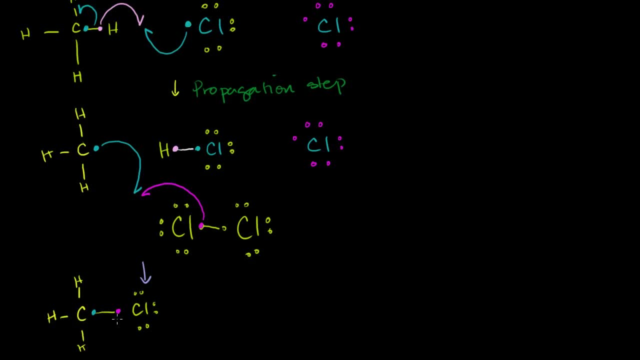 valence electrons. They are now bonded. This is chloromethane, And now you have another free radical, Because this guy- and I should have drawn it there, this guy, the bond was broken, So he gets back his electron. 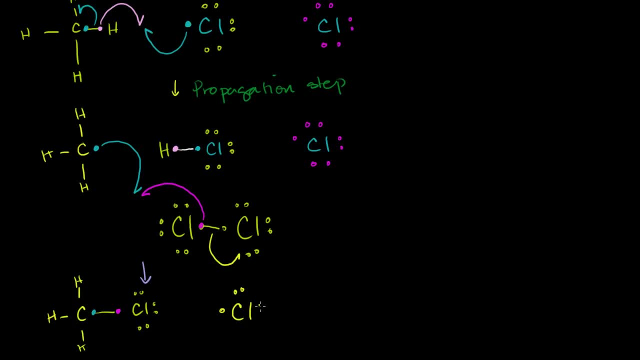 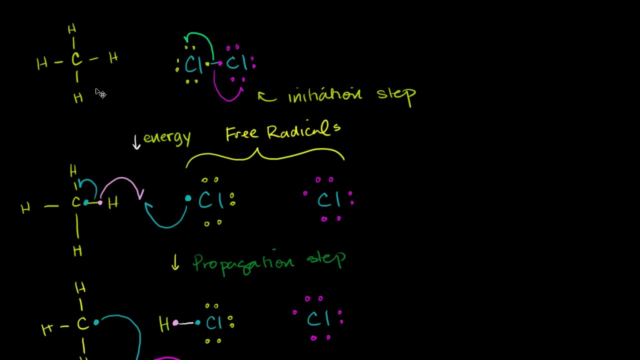 So he's sitting over here. He is now a free radical, So this is another propagation step, And we still have that original free radical guy sitting out over here. So we keep forming more and more free radicals. as this happens, Now, eventually we're going to start running out of methane. 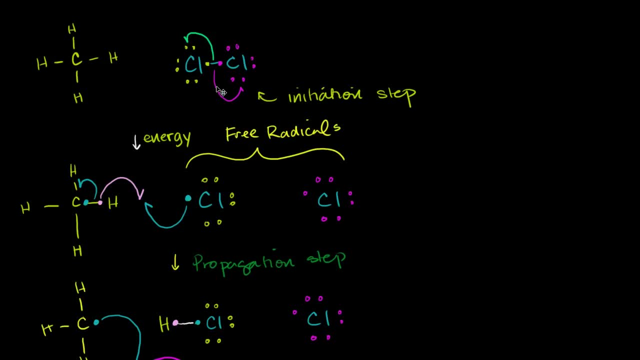 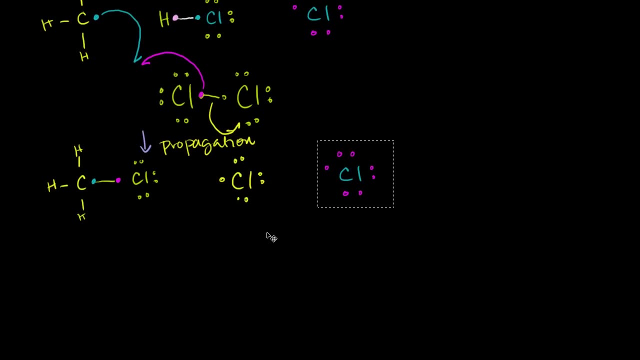 We're going to start running it, running, Running out, So they're going to be less likely to react and you're actually going to have more free radicals around. So once the concentration of free radicals gets high enough, then you might start to see them reacting with each other. 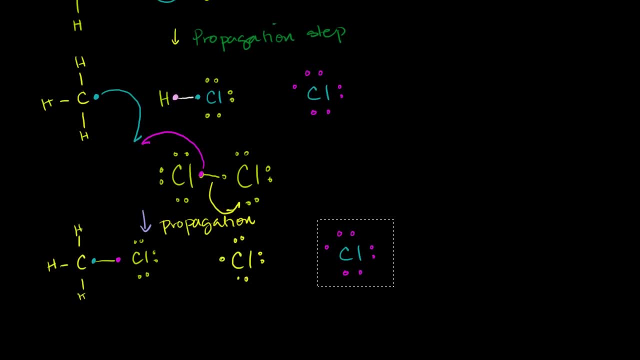 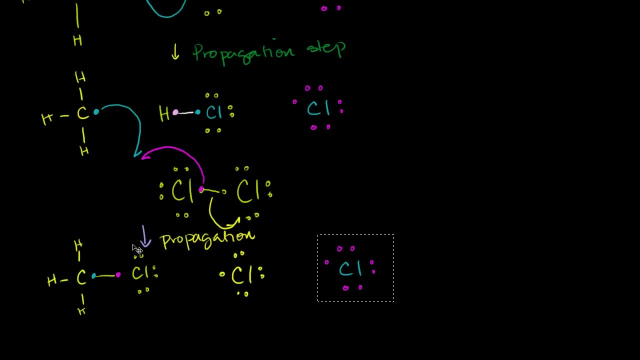 So when the concentration of free radicals get high enough, you might see, instead of this step happening, this will happen a long time until most of the free radicals or most of the non-free radicals disappear. but once we have a soup of mainly free radicals, you'll see things like this: 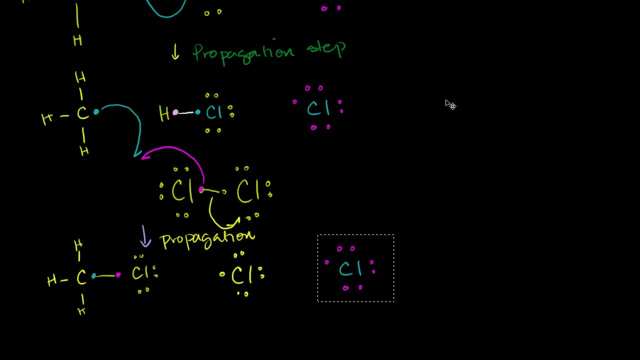 You'll see the methyl free radical, so let me draw it like this: you'll see him maybe reacting with another methyl free radical, with another methyl free radical, where they both contribute an electron to form a bond, And then, once the bond forms, you have ethane. 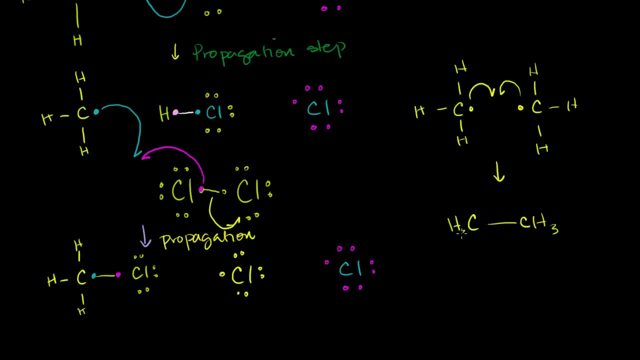 I could just write it as CH3. H3C. So you might have something like this. And so this type of a step where two free radicals kind of cancel each other out. this is a termination step, because it's starting to lower the concentration of free radicals in the solution. 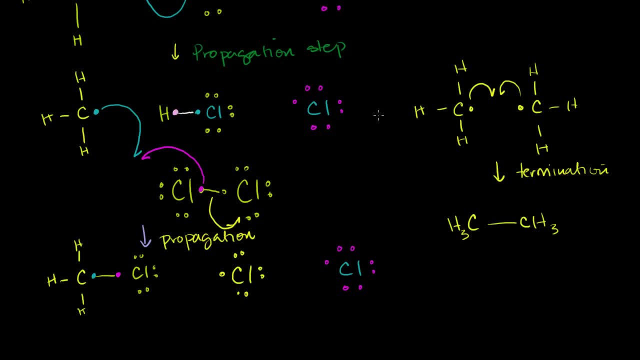 But this is only. once the concentration of free radicals becomes really high, You might also see some of the chlorines cancel out with each other again. So a chlorine free radical and another chlorine free radical. I'll only draw the unpaired electron. They can bond with each other and form molecular bonds. 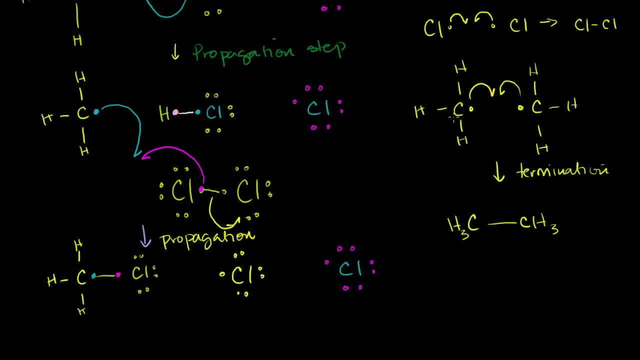 So they're chlorine again. That again is a termination step. Or you could see something like the methyl free radical. Let me just just for shorthand I'll write it like this: H3C, The methyl free radical, and a chlorine free radical might also just straight up react and form chloromethane. 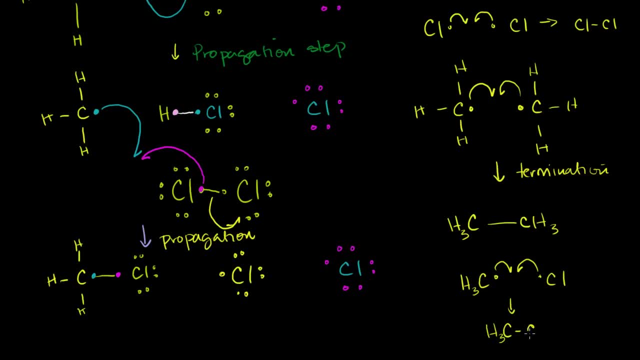 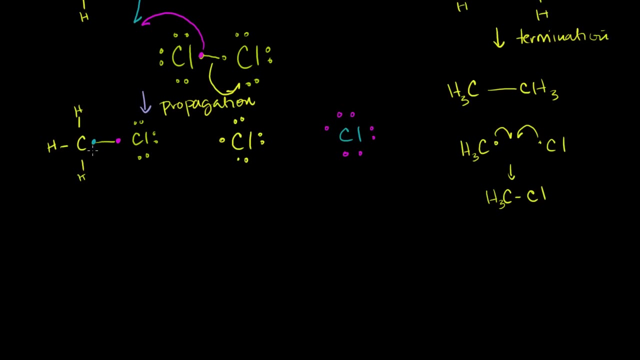 And form H3CCl. So this will all happen once the concentration of free radicals gets really high. Now another thing that might happen if this reaction proceeds- we have a lot of the propagation steps- is that you might have a situation where you already have a chloro. 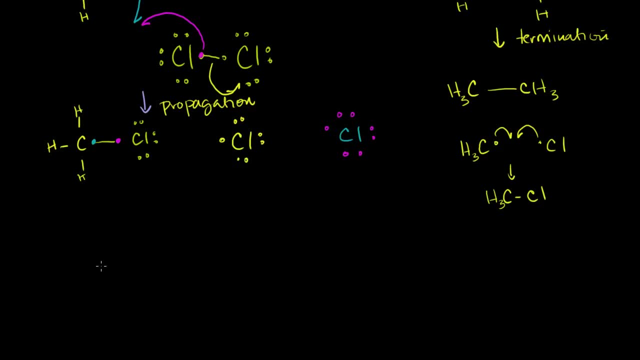 you already have a chloromethane. You already have a chloromethane, So it looks like this: You already have a chloromethane, And once you have enough of these, it then becomes more likely that some free radical chlorine 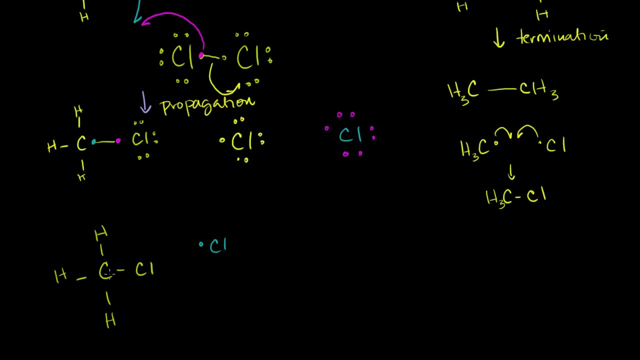 that some free radical chlorine might be able to react with this thing. So it might. it might actually add another chlorine to this molecule And the way it would do it this chlorine over here I'm just drawing the free electron pairs. 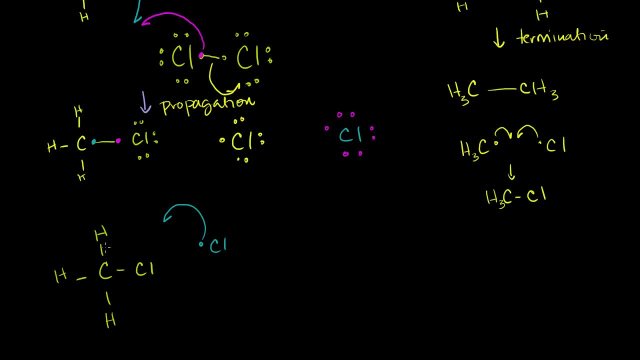 It would form a bond. it would form a bond with this hydrogen right over there. They would both contribute their electrons And then the carbon would take back its electron. The carbon would take back its electron. Notice all the half arrows. And then we'd be left with 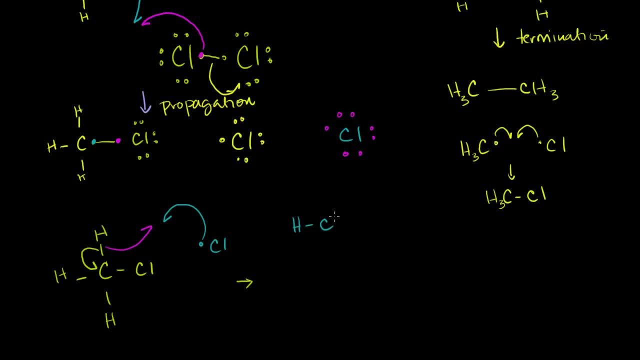 you'd be left with the hydrogen and the chlorine would have bonded. And now this guy is going to be a free radical, But he's going to be a chlorinated free radical, So it's going to look like this. Let me see.